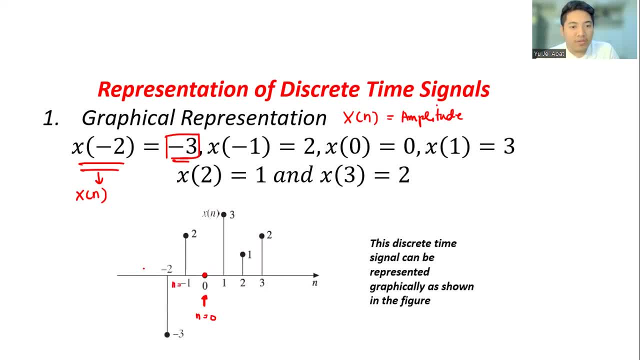 You also have n equal negative 1.. You also have n equal negative 2.. So if we're going to represent the signal x of negative 2, with a value of negative 3. So it means the position is in negative 2 of the n and its amplitude is negative 3.. 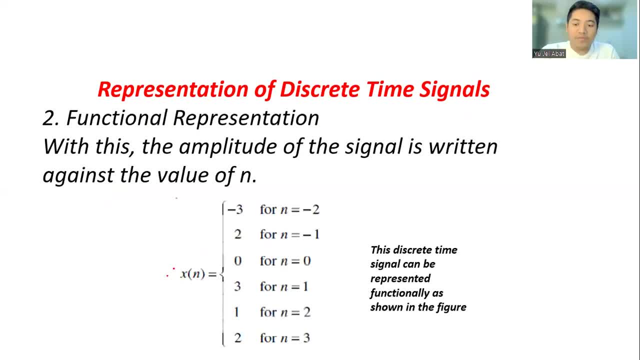 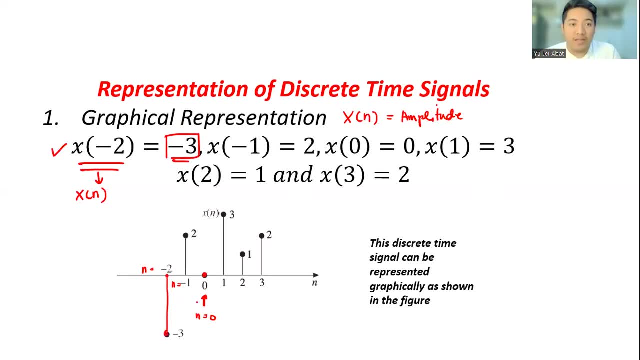 So that we will be having this kind of signal here. So we have this kind of signal here for the position x of negative 2.. And the same as with the x of negative 1, we have a value of the amplitude of positive 2,. 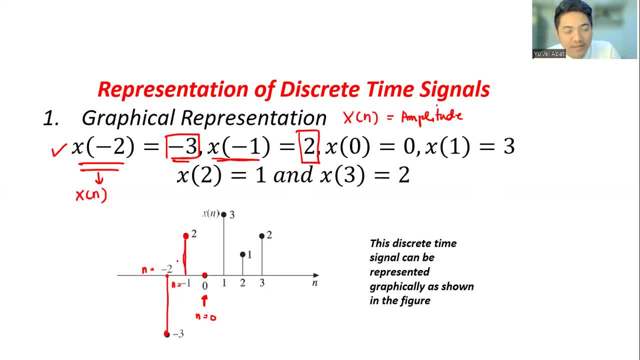 so that we can represent that discrete time signal. So that we can represent that discrete time signal in this one x of zero equals zero, So we have a value of zero. in the n equals zero, So we have x of 1, amplitude of 3.. 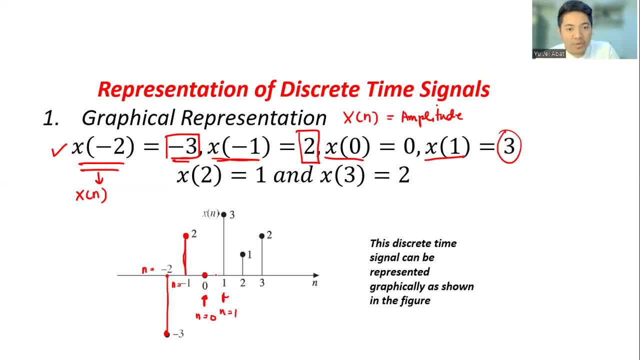 So we have the position for n equals 1,. okay, Its amplitude is positive 3.. So we have here, as x of n amplitude of 3, and we have x of 2. So position is 2, and, of course, the value of n is 2.. 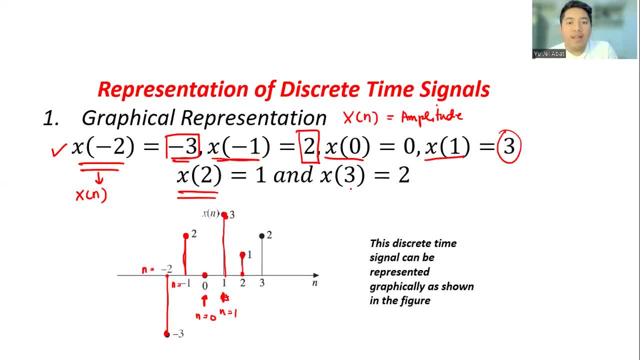 Then we have a value of the amplitude as 1.. And, last but not least, we have x of 3.. So we have the value of 2 as an amplitude. So this is the discrete time signal represented by graphical representation. Okay, so that's one way of representing discrete time signals. 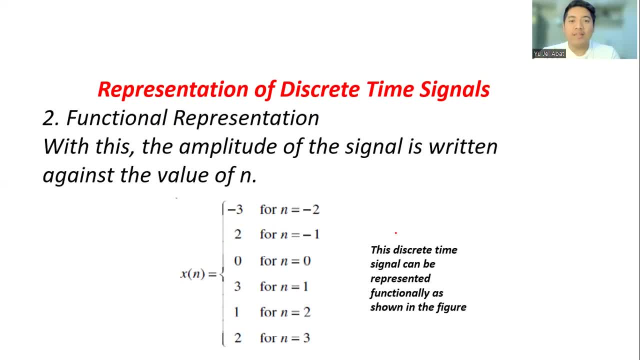 Number two: we have functional representation. So with this the amplitude of the signal is displayed here For every value of x, of n, for the corresponding position n in the axis. So the amplitude of the signal is written against the value of n. 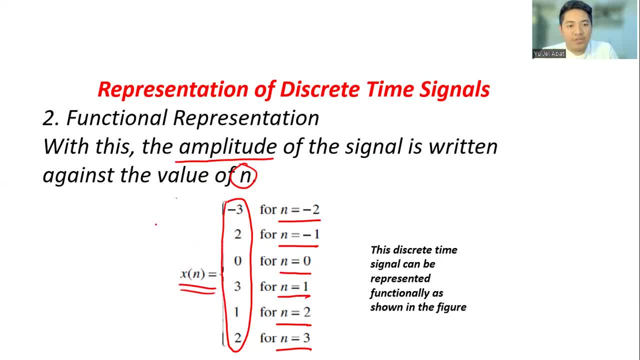 So it means that its function is x of n, So with a values of the amplitude here. So here are the amplitude. So meaning if we have x of negative 2, for negative 2, x of n, so we have a value of negative 3.. 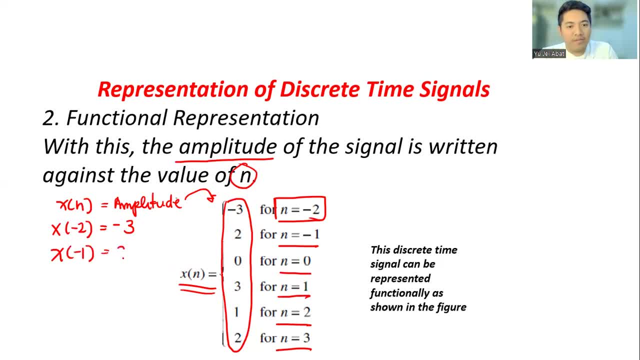 So for a value of x, of negative 1, so we have a value of 2 as amplitude, and so on and so forth. So this discrete time can be represented functionally. So you may also get a function that is piecewise function. 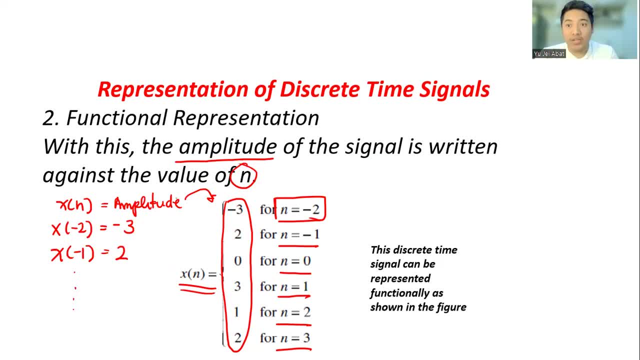 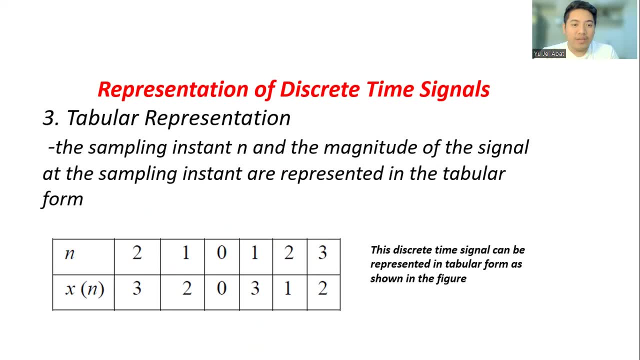 Okay, if we are representing functional representation. Tabular representation is another statement, Straightforward Okay, representation of the signals that we have, of course. So, correction: this is only negative 2.. And so we have negative 2, negative 1 here. 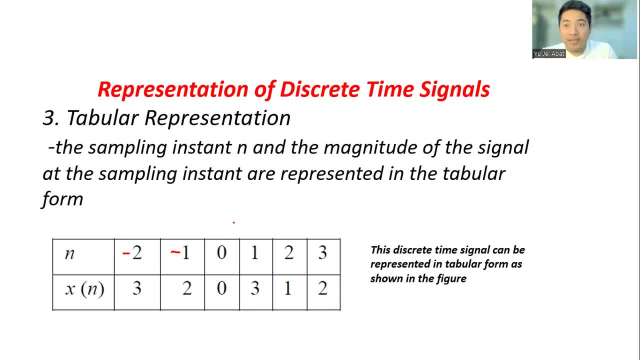 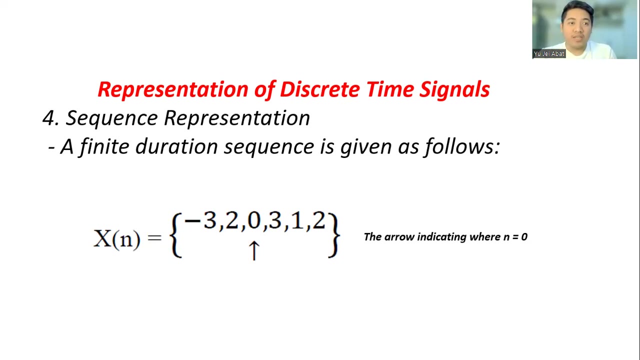 So, because the position of n indicates the position of the signal in the axis, So tabular representation. Okay, These are the amplitude, These are the position, So same representation. Also, the sequence representation is one of the most used representation of discrete time signals. 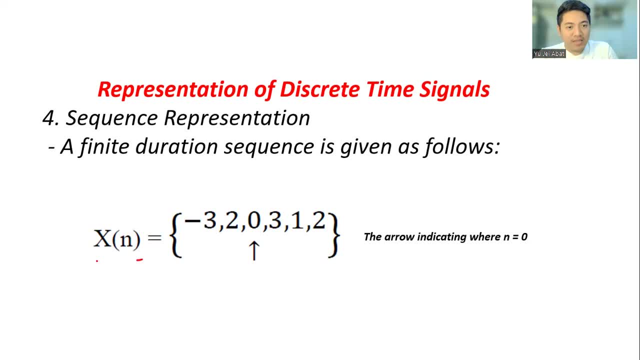 So a finite duration sequence is given as follows: So you have x of n, followed by a bracket. So we have, these are the values of the amplitude. Okay, these are amplitudes. Right, And we have, If we can. we can notice we have an arrow there that denotes that n equals zero. 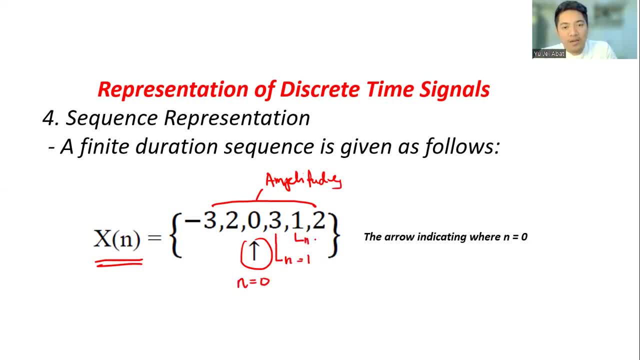 So this will be your n equals 1,, n equals 2, and n equals 3.. So on the left side, of course, this would be your n equals negative 1 and this would be your n equals negative 2.. So that's how you represent discrete time signal in the sequence representation. 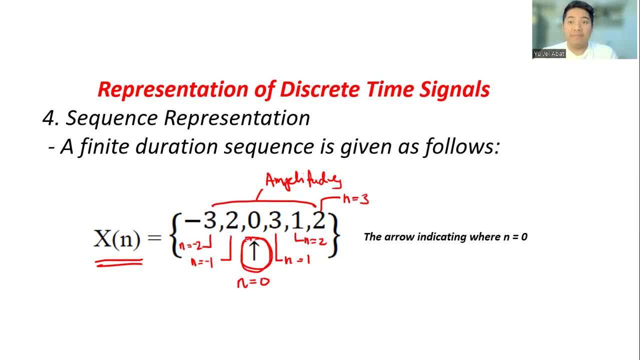 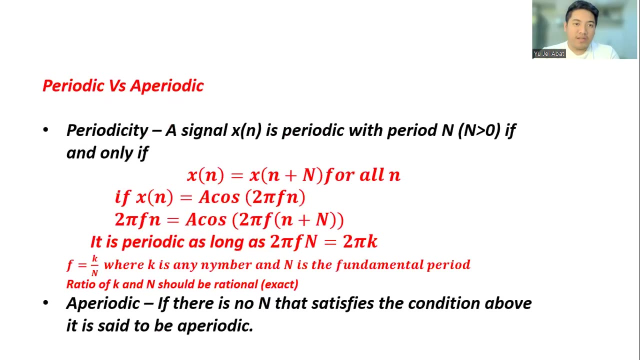 So if we see an arrow here, it represents that the signal On that specific time, On that specific value of amplitude is set at n equals zero. So the arrow indicating where the n equals zero. So we also have one property of signals. 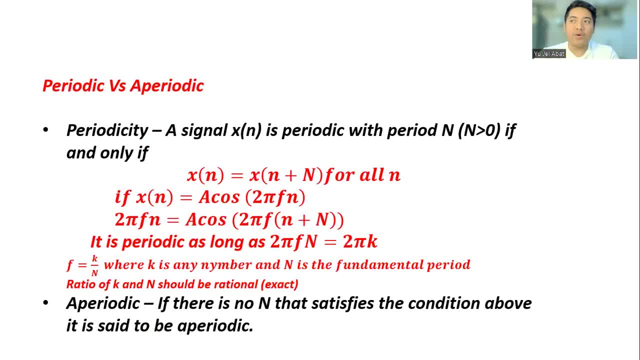 So we have periodic and aperiodic. So when we say aperiodic, the certain signal repeats at a certain period n. Okay, So we say that a signal is periodic if the signal x of n is periodic with the period n. where n is greater than zero, n is the period. if, and only if, the value of x of n, or the signal equals f, equals x of quantity n, which n is any number plus the period. 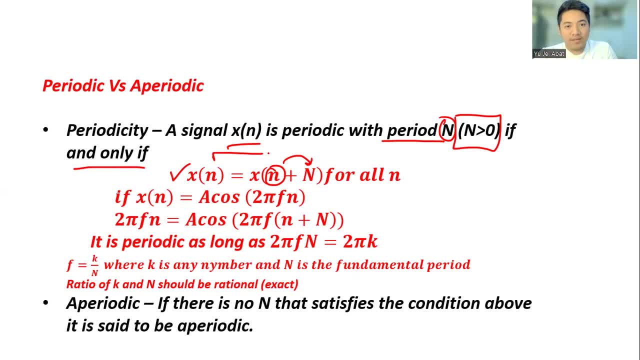 So if we, if these two equates, okay, we can conclude that the signal is periodic. But if the given signal is in terms of, let's say, Cosine or sinusoidal wave, So if x of n equals a, where a is the amplitude cosine of 2 pi fn, of course this 2 pi fn denotes the angular frequency, right? 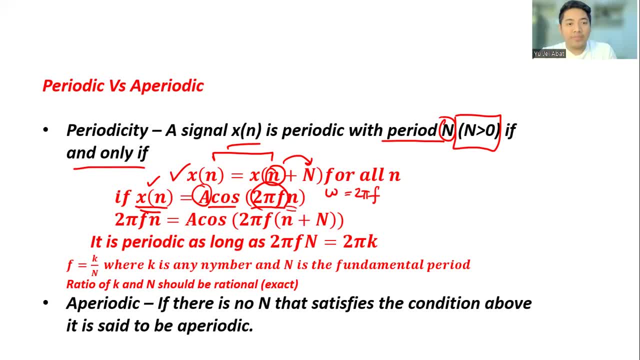 So 2 pi fn, then it is periodic. if 2 pi fn equals a cosine, 2 pi f, okay, quantity n plus n. So we can notice here that the value of n- here the smaller n, Lower case n, is added by another big letter, n, which is the period, which is, which is actually the same thing we applied here, because that's the condition. 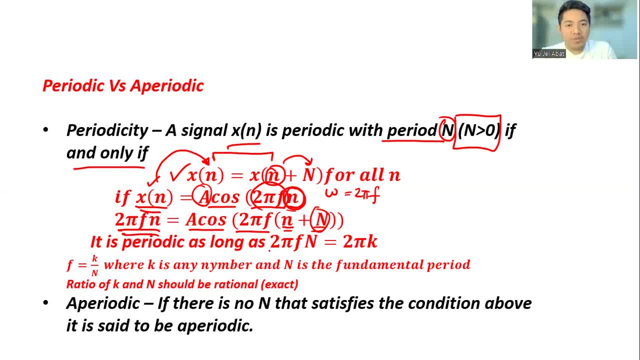 Okay, So it is periodic, as long as the 2 pi fn, together with the period, equals the 2 pi k. Okay. So, anyway, later on we will understand how to solve those equations, So resulting in an f Okay Equals. 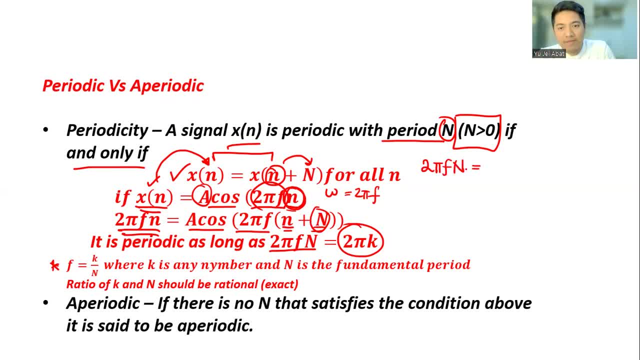 Okay. So if we are going to equate this, 2 pi fn equals 2 pi k, where k is any real number and n- upper case n- is any the period itself. So we can notice that the 2 pi's will cancel and we have frequency. 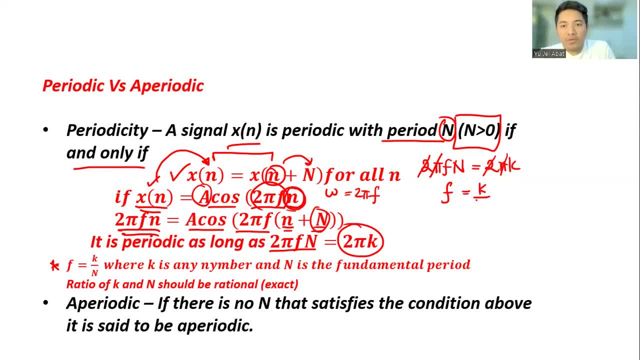 If we isolate frequency, it can result to k all over n, where k is any number And your n is your Period. Okay, So we can say, okay that the signal is periodic. If the value of n is an exact ratio, okay, n should be a rational value. 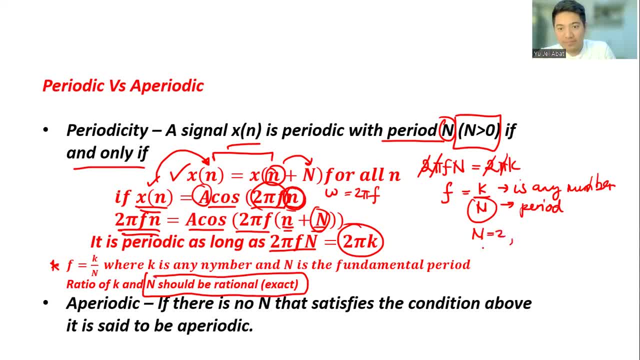 Okay, Exact. So if n is 2,, okay, upon figuring out the f all over k, all over n, if n is 2, if n is exact 4, if n is equal to 6,, n equals 12,. these are exact number. 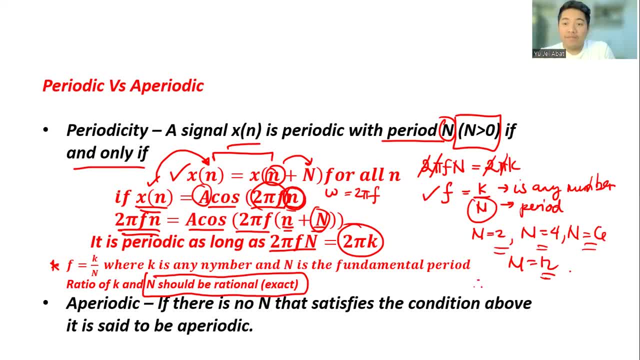 So it is said that this is periodic, While if the value of n becomes 2 pi, okay, value of n becomes 3 pi. So that's irrational. We conclude it as a periodic. It does not repeat itself over the process of a certain period. 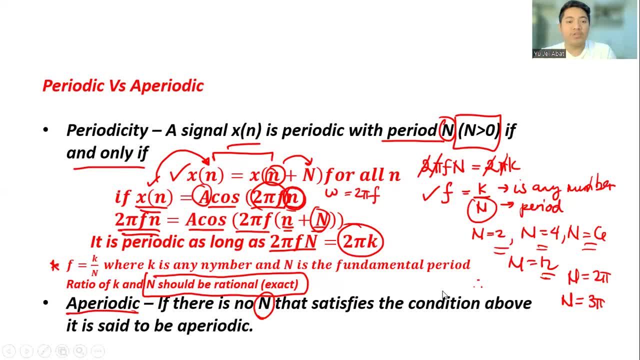 Okay, If there is no period that satisfies the condition above, it is said to be a periodic, So let us try. Let us try to solve some examples. okay, to test the periodicity and a periodicity or periodicity of the signal. 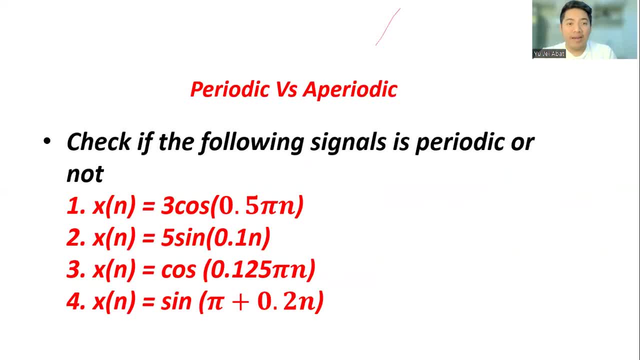 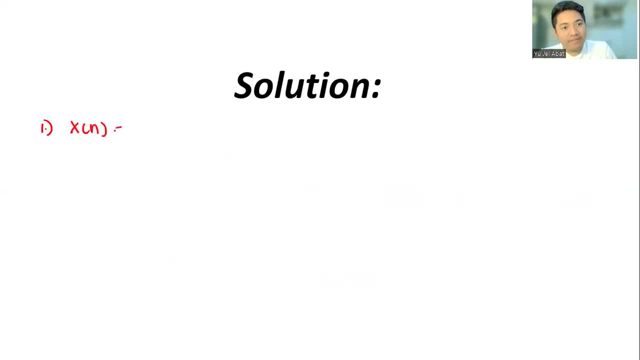 So check if the following signals is a periodic or not. So let us start first with the first number, That is: x of n equals 3 cosine of 0.5 pi, n. Okay, So the very first thing is that, Okay. 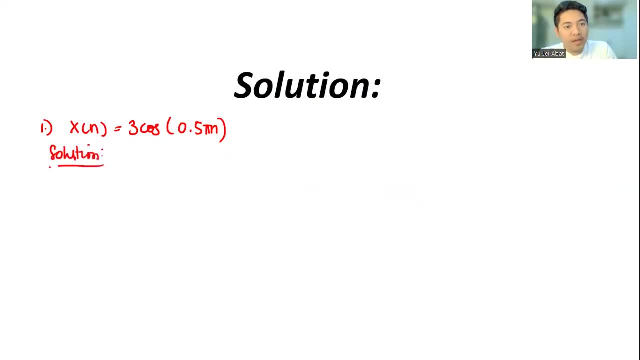 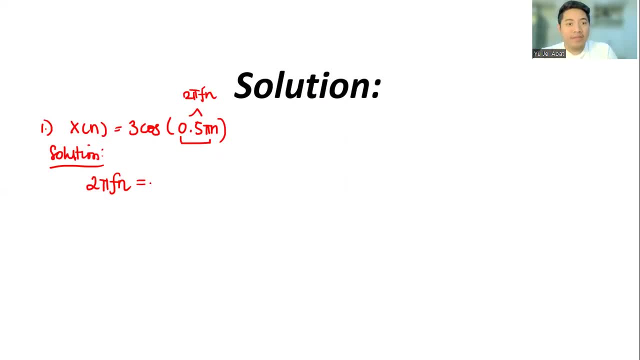 What is the 2 pi fn to get the frequency. So we have 0.5 pi n And this 2 pi, or I mean, sorry, okay, 2 pi fn and 0.5 pi and this n will cancel, the pi will cancel. so you have, you are left with 2f equals. 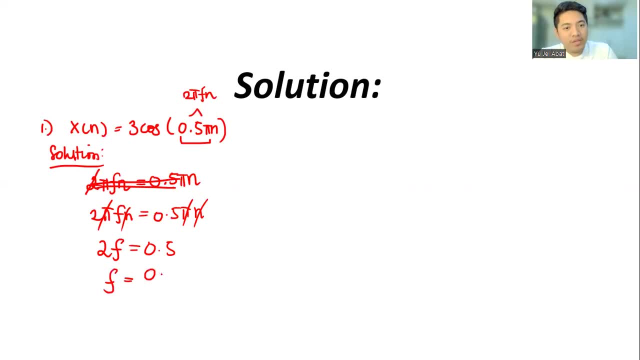 0.5 here. so the frequency would be 0.5 all over 2 and remember our formula is k all over n. where k is any integer, okay, and if the n is rational or exact, okay, that's the period- then it means that it is periodic. so in this case, if we simplify this using our calculator, of course that's 0.25. 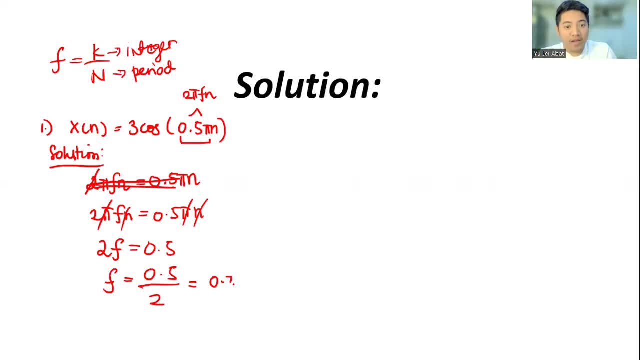 but the fractional part of 0.25 is what? okay, the fractional part, that is one fourth, okay, so this is your k. okay, so this is your k, okay, so this is your k and this is your fundamental period. so it means that this signal has a period of 4, which is an. 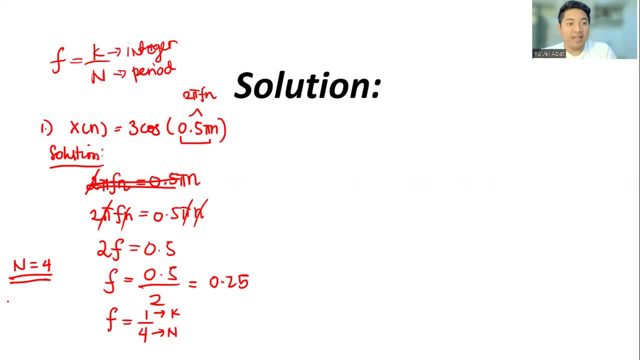 rational, irrational number, exact number. so therefore we conclude that this is periodic. okay, so that's periodic. that's for number one. so for number two we try to solve again the problem. so we have x of n, we have x of n, we have 5 sine of 0.1n. so what are we going to do? again, get 2 pi fn, that would be 0.1n. 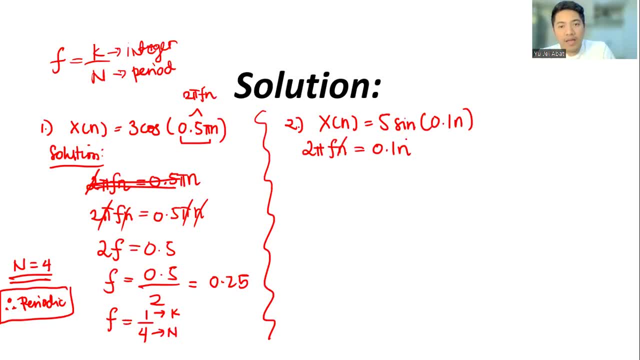 so, as you can see, the n will cancel. so you are left with 2 pi. f here equals 0.1. get the frequency by dividing both sides by 2 pi, so you have 0.1 all over 2 pi. so this will be your k, and then you. 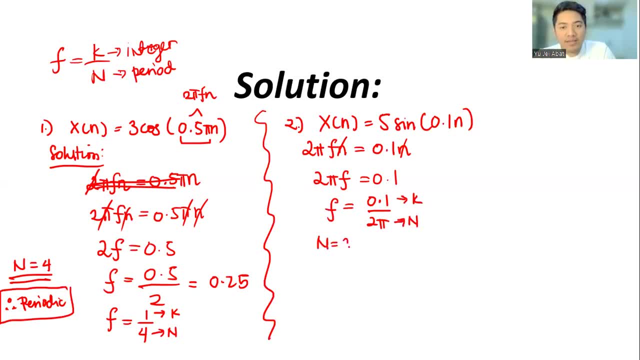 and this will be your n. so your n in this case is 2 pi, which is irrational, not exact. if you evaluate 2 pi, that's around uh, 6 point, something right? so therefore, our signal x of n is a periodic. okay, that's the number two. 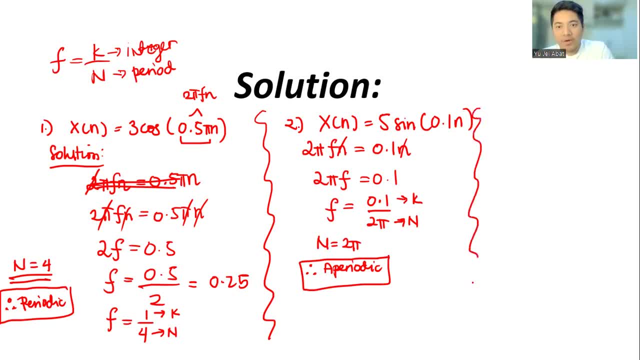 okay, so how about for the next one? we're going to do the next one, we're going to do the next one, number three. so we have x of n equals sine or cosine of 0.125 pi n. okay, so again, 2 pi fn. we want to get the frequency or the ratio of the k all over the period. so we have 0.125 pi n. 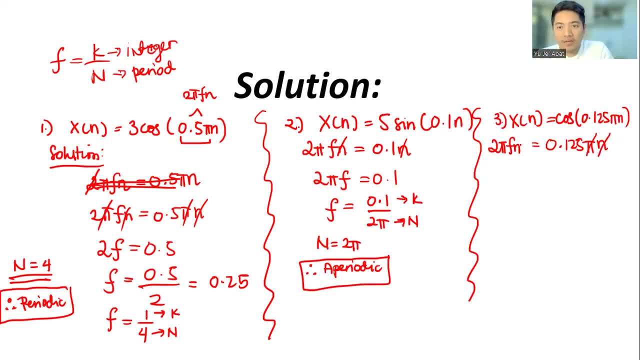 okay. so, as you can see, the pi n will cancel. okay, so pi and n. so we have 2 f, twice the frequency, all over 0.25. so divide both sides by 2, so we have 0.125 all over 2, which is what? if you're going to evaluate that, that will be 1 all. 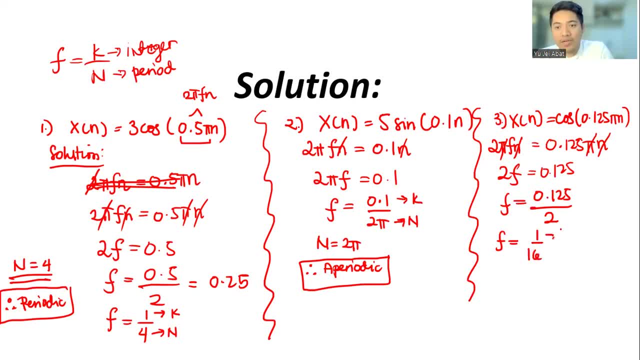 over 16 in fractional form. okay, so this is your k and this is your period, fundamental period. so we have n. okay, equals 16. okay, so this is your k and this is your period, fundamental period. so we have n. okay, equals 16. okay, so divide both sides by 2 so we have 0.125 pi. n, so we have 2 pi and n, so we have. 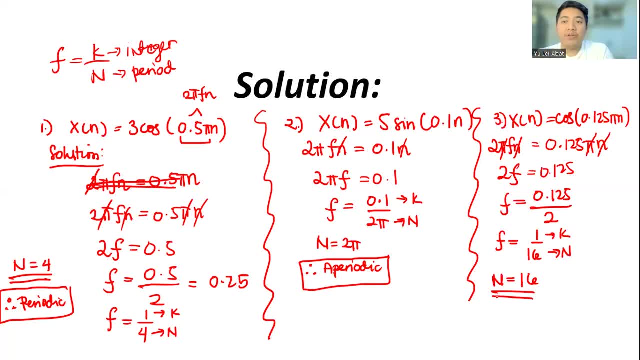 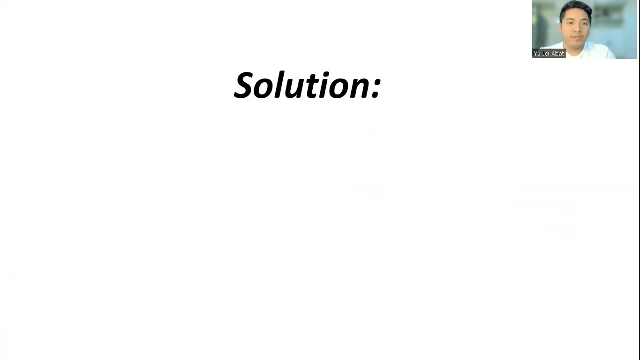 So it means the value of n or the period is rational, exact. So therefore, this signal is periodic. Okay, so that will be periodic. Okay, so that is for our number 3.. So how about if- for number 4, we have a signal that has a complex sum of, let's say, a real number with e, j pi n all over 12, plus the imaginary, or the sum of this real number and this imaginary e raised to j pi n? 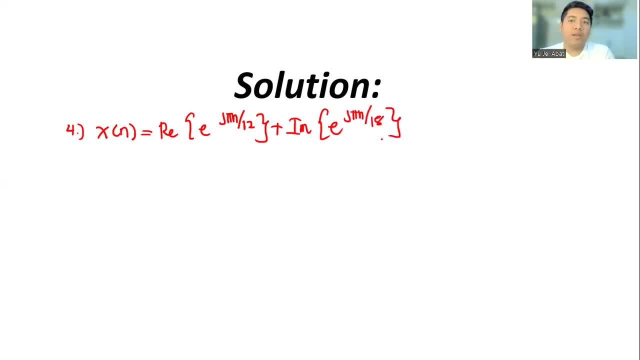 So we can recall that from our sinusoids or Euler's identity, that we can resolve this into sum of cosine and sine. So we can rewrite this as x of n, as the cosine of pi n all over 12, plus we have the sine of pi n all over 18.. 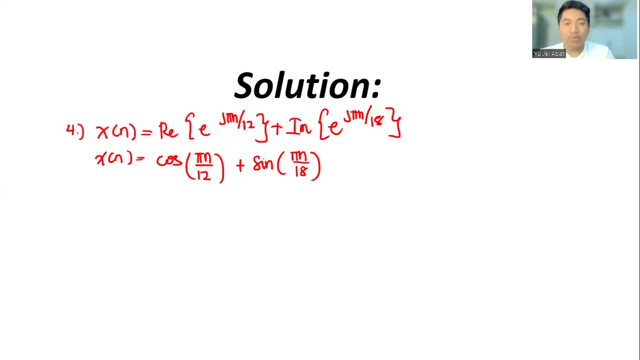 Okay. so now we have, If we have two sinusoids, Okay. if we have these two sinusoids added, okay. if we want to determine the fundamental period, okay. so we're going to determine only the fundamental period, But we will also see later that these two sinusoids have a period or periodic function because of the rational value of the value of n. 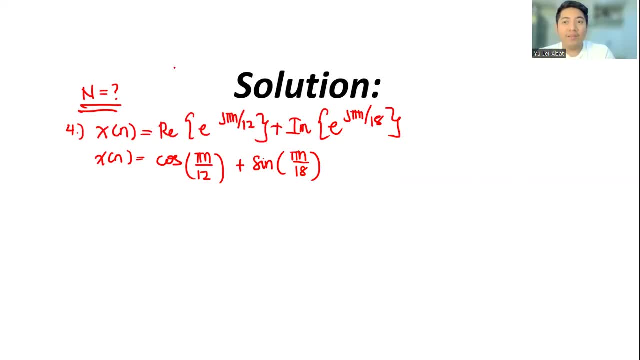 So to find, So to find the fundamental period, fundamental period of these two added signals. so we're going to use the formula: n equals n sub 1, where n sub 1 is the period of the first signal multiplied by n sub 2, all over, which is the period of the second signal all over. gcd of n sub 1 and n sub 2, greatest common divisor. 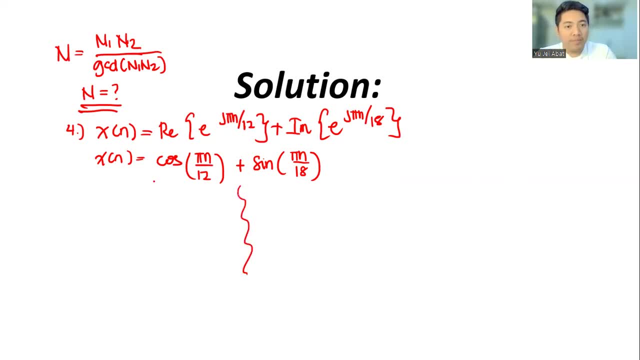 So the first I'm going to get for the period of cosine part. So we have 2 pi fn equals pi, Pi n all over 12.. So cancel n and then pi, So we have 2 f equals 1, all over 12.. 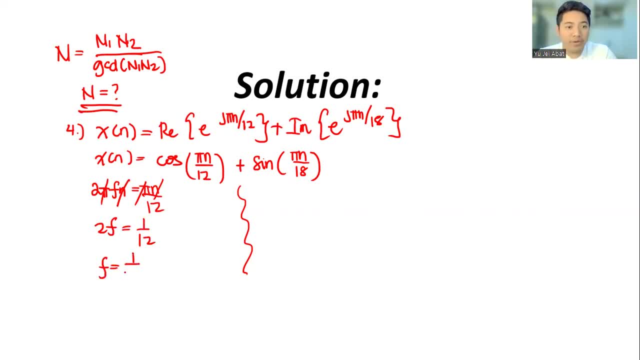 Getting the frequency, or the fundamental frequency or the fundamental period. we have 1 all over 24.. Okay, because of dividing it by 2.. So this is my k and this is my n sub 1.. Okay, so my n sub 1 is 24, which proves that this is a periodic signal. 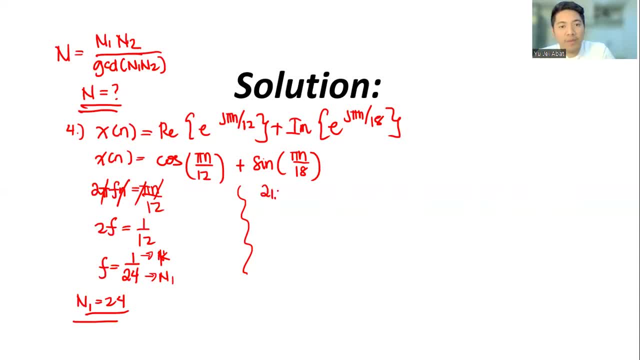 So another one, Another sign: we have 2 pi fn. Okay, we have pi n all over 18.. So cancel is pi n. So you have 2 f equals 1 all over 18.. But if we're going to divide it both sides by 2 or cross multiply, so you have 18 times 32 is 36 divided by 36, you will be having f1 all over 36, where this is your k and this is your f. 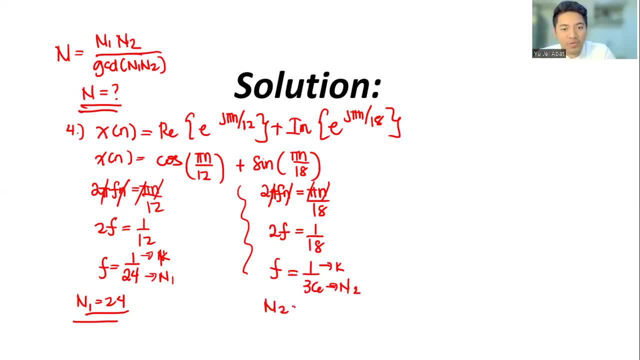 Okay, So this would be n sub 2.. So your n sub 2 would be 36.. Both are exact, rational, So to get the fundamental frequency. So our problem here: what is the Not frequency? I'm sorry. 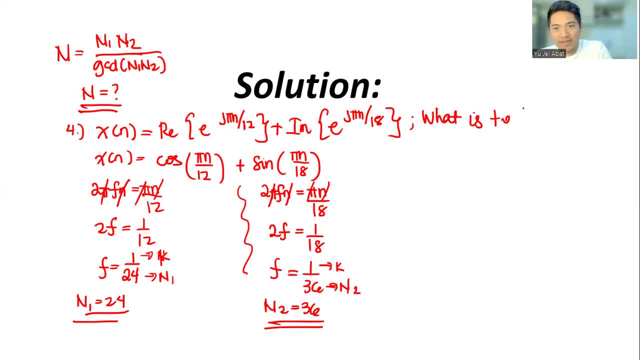 The fundamental period. What is the fundamental period of the sum of these two sinusoidal? So, by the way, this formula- Okay, Okay, Okay, Okay, Okay, Okay, Okay- Also applies to multiplication of two sinusoidal. Not only plus, but in our example it's plus. 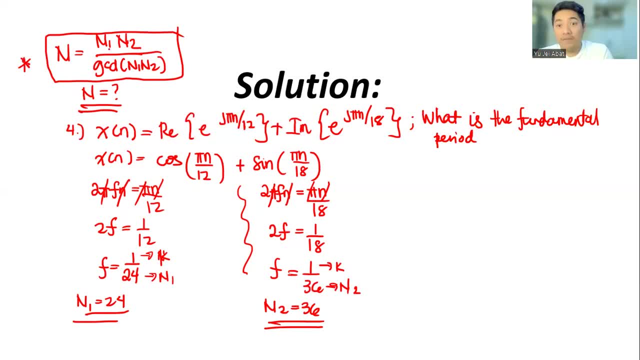 And as well as multiplication, we can apply this formula. So what is the fundamental period? The fundamental period would be n1 times n2, all over the GCD of n1 and n2.. Okay, So we have n equals n1 will be 24.. 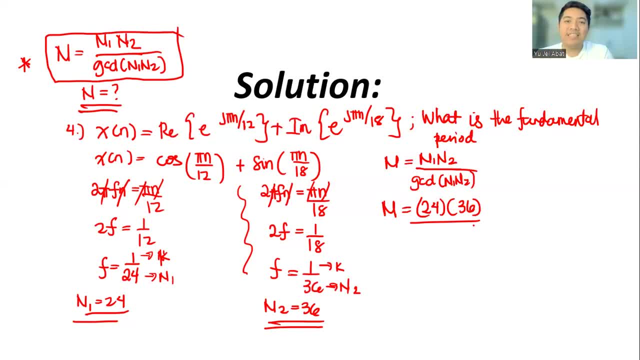 And we have 36. All over, what is the GCD? What is the greatest common divisor of 24 and 36?? So it would be 12.. Okay, So that's the greatest common divisor of between the n2 and n1.. 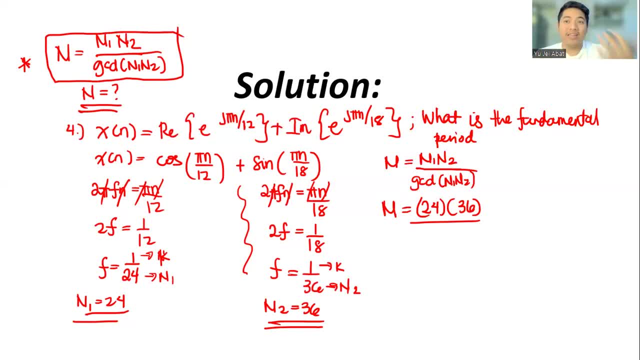 So 12, because it's the nearest divisor that we can divide: 2.. Okay, The two periods: 24 divided by 12 is 2.. 36 divided by 12 is 3.. That's the greatest common divisor, Okay. 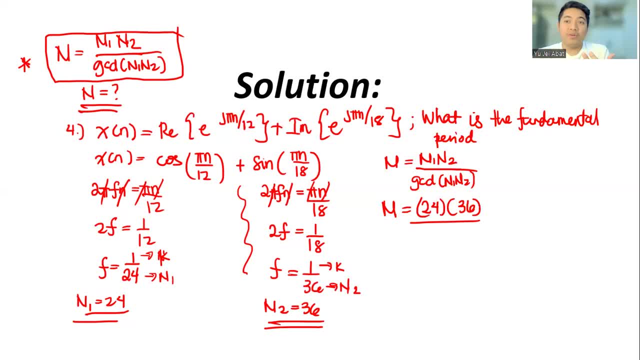 It's not 3.. Because they can be divisible also by 6. They can be also divisible by 6.. 9, it's not divisible because 24 is not divisible. So that's not the greatest common divisor, But 12.. 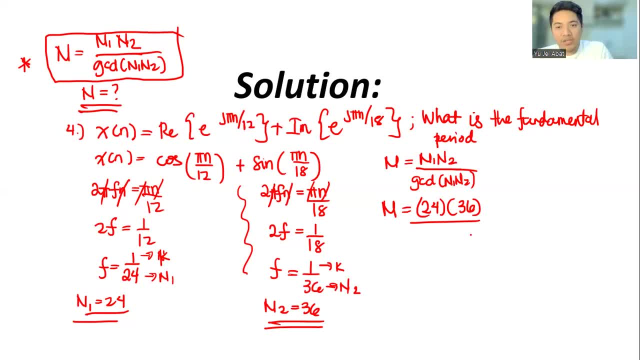 Okay, So 12, 24,, 12,, 24,, 36.. So it becomes a 12.. So, upon calculating the basic or the fundamental period of that would be 72.. Okay, Okay, So that is how we are going to compute the fundamental period of that signal. 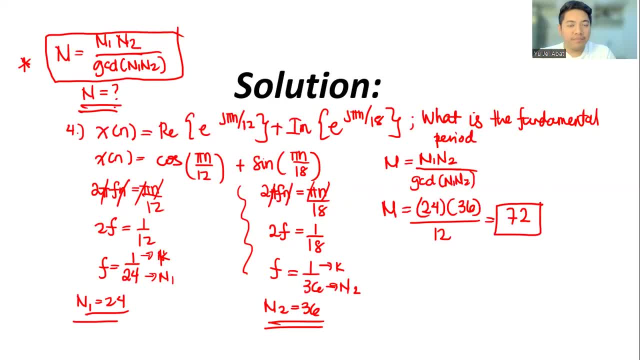 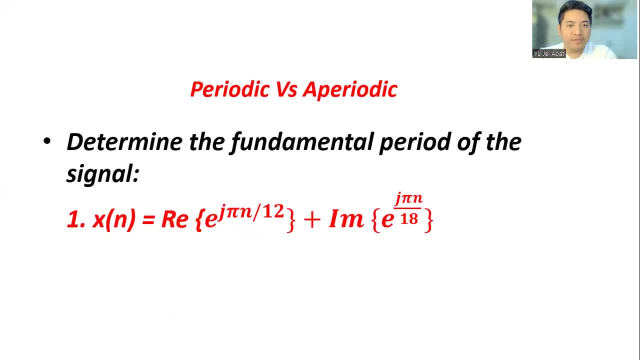 So how about in number 5?? Okay, So that's the example a while ago. So for number 5, let's example for this. By the way, you have x of n, e raised to j, pi, n, all over 16.. 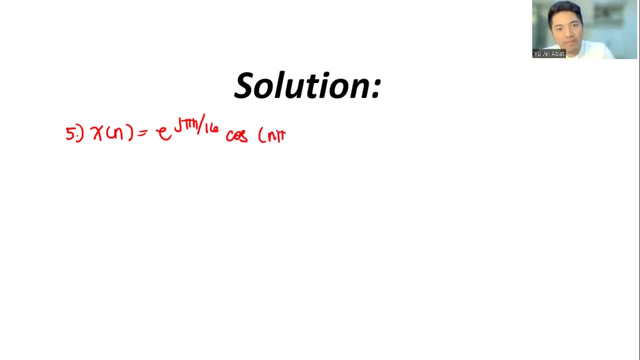 That would be multiplied by cosine of n- pi- all over 17.. Okay, So this is multiplication. So we have here e raised to j- pi- n all over 16.. We have cosine here, So actually we can get the value of. 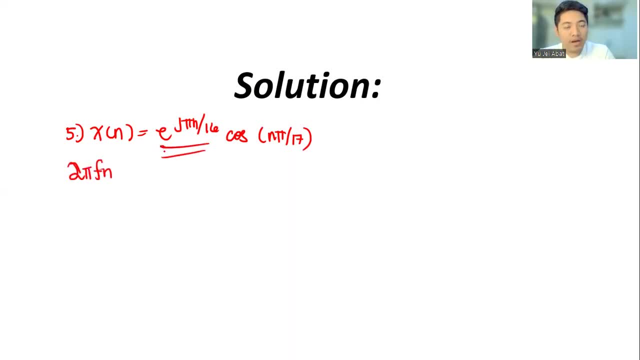 So we have 2 pi fn first of this signal. So we have pi n all over 16.. So pi and n will cancel. So you have 2f all over 1,, all over 16.. So our frequency will over 1,, all over 32, which is: this is your k and this is your n1.. 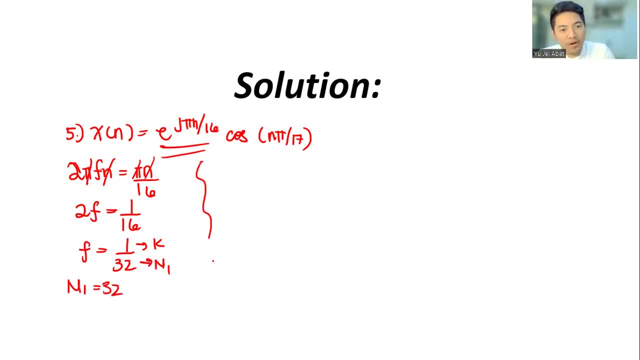 So your n1 will be 32.. On the other hand, computing for the cosine, we have 2 pi fn, So we have 2 pi fn. The period, So n pi will cancel both sides. So we have 2f equals 1 all over 17,, which is 1 all over 34..